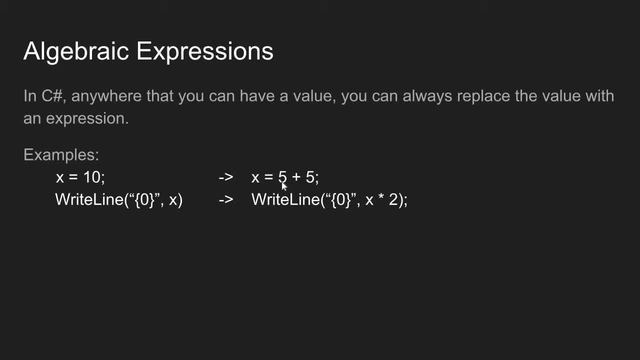 happens. here is before I can do the assignment. this expression has to resolve into a value. So 5 plus 5 equals 5.. would resolve into the value 10, then I could add 10 or assign 10 into X. Let's look at another. 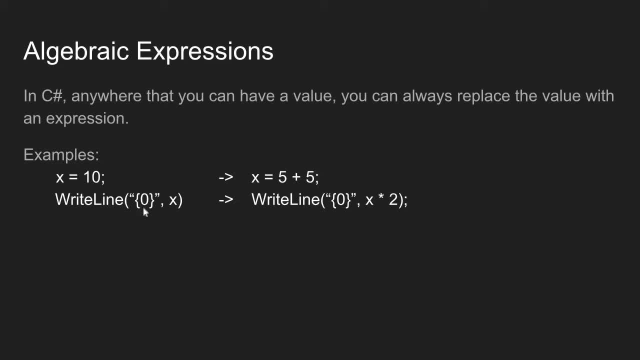 example, Here I'm calling the right line method and I have some formatted string and I want to insert a value into that string, so some value X. Well, I could replace the value with an algebraic expression: X times 2.. So in this case, before I can insert this value into my string, so I can 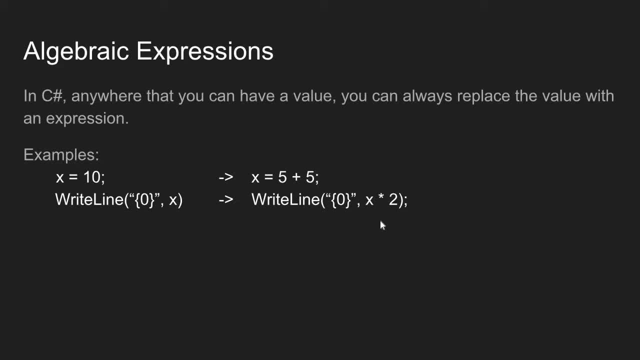 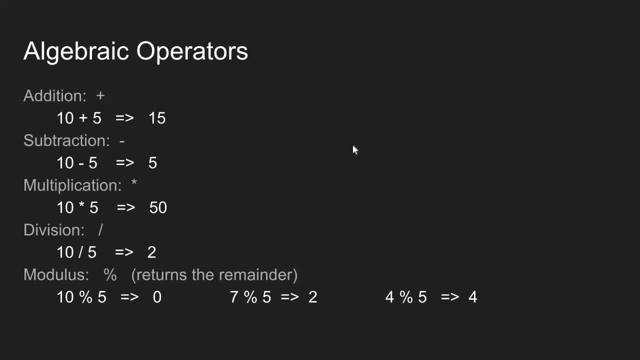 print it. this expression has to resolve to a value, So we would have to do the math, or the compiler would do the math, come up with a result, then I could insert the result into the right line. So here are our five basic algebraic operators. The plus sign is the addition operator. 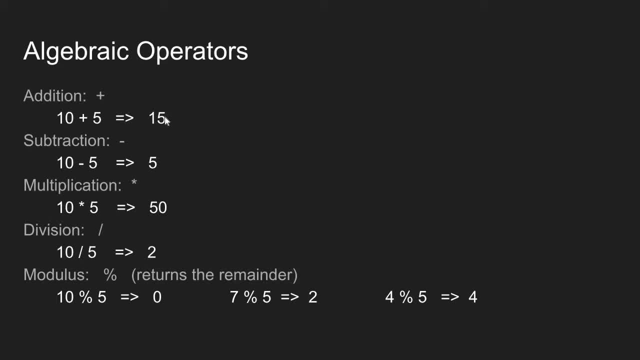 It adds two values. So 10 plus 5 would give me the value 15.. The minus sign is the addition value. So 10 plus 5 would give me the value 15.. is the addition value. So 10 plus 5 would give me the value 15.. 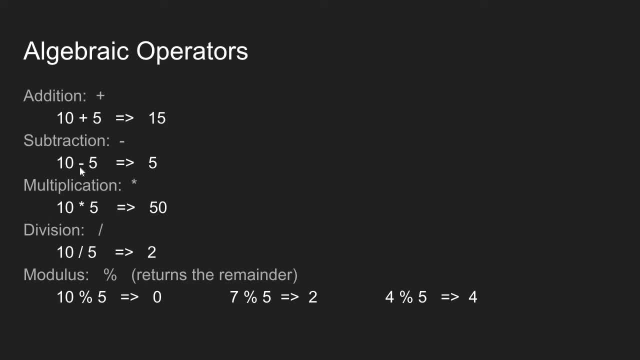 minus operator subtracts values. So 10 minus 5 would give me the value 5.. We are subtracting 5 from 10.. The multiplication operator is an asterisk. So 10 asterisk 5 stands for 10 times 5.. When we multiply 10 by 5, this gives us the value 50. And then the division operator is a. 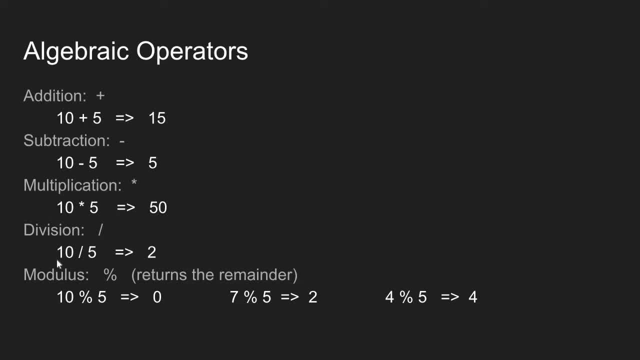 forward slash, a single forward slash. So 10 divided by 5 would give me 2.. Now the new operator that you may not be aware of is the modulus operator, And it's the modulus operator. in C, sharp is a percent sign. The modulus returns the remainder when you divide one value by another. 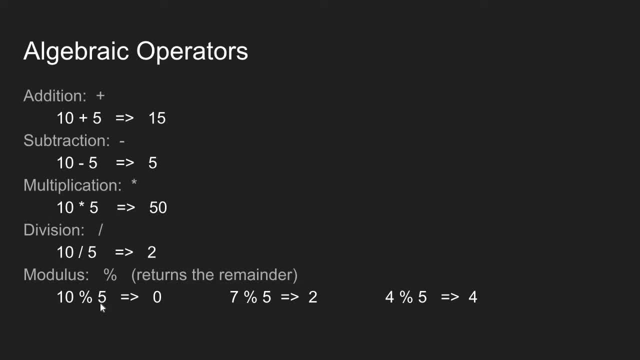 So, for example, 10 modulus 5 would return the result if I divided 10 by 5.. 5 will go into 10, two times with 0 left over. So the remainder is 0.. So 10 modulus 5 returns 0.. 7 modulus 5, if I 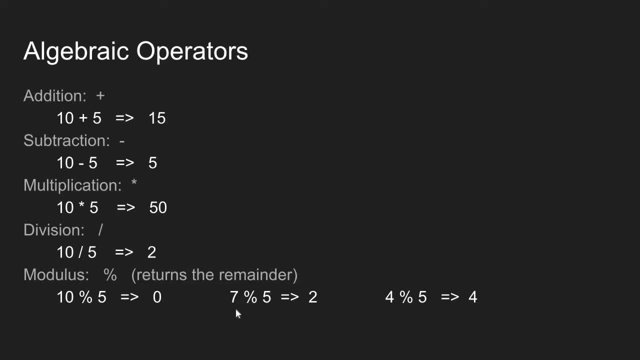 take 7 divided by 5,, 5 will go into 7 one time, with 2 left over the remainder of 2.. So 7 modulus 5 returns 2.. We return the remainder 4 modulus 5,. if I were to take 4 and divide it by 5., 5 will 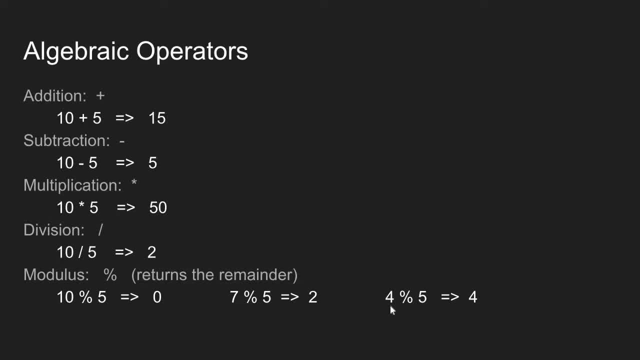 go into 4 and divide it by 4.. So the remainder is 0.. So 10 modulus 5 returns 0. So the remainder is 0 times with 4 left over. So 4 modulus 5 would produce the value 4.. So modulus is. 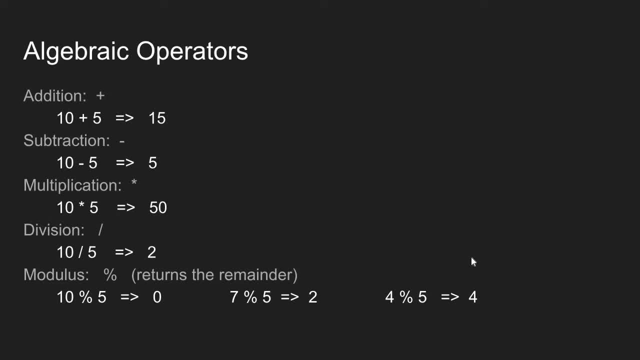 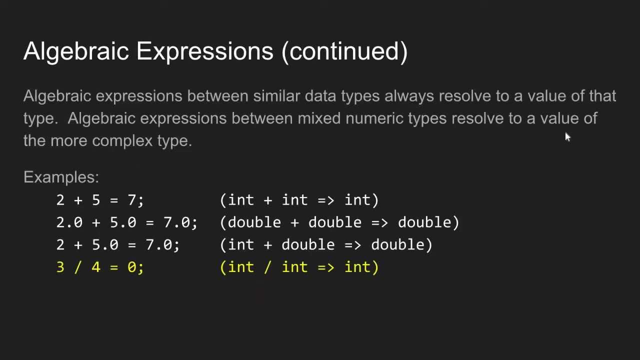 a is a useful operator. It helps you do a lot of interesting tricks when you're coding. It's a good one to learn. Alright, when you use an algebraic operator between two similar data types, the result that it produces is always that. 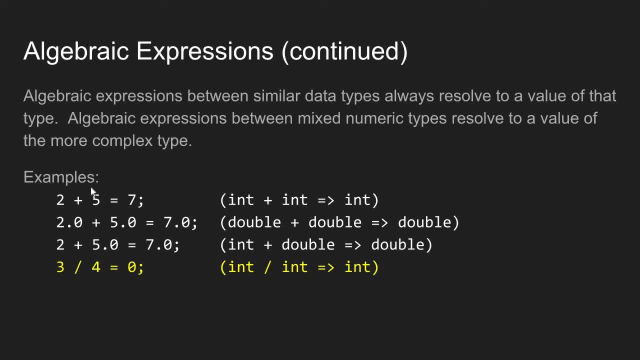 data type. So, for example, an int operating against an int will always produce an int Double operating with a double will always produce a double. Algebraic expressions between mixed data types always give you the more complex type. So if I have an integer 2 and I'm interacting with a double 5, the result 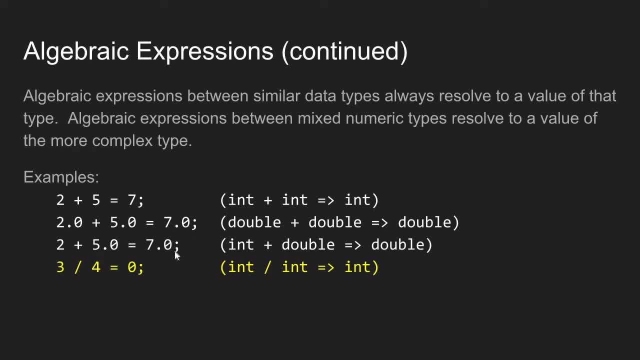 that it produces will be a double. It's the more complex type. So again, integer 2 plus integer 5 gives me integer 7.. A double 2 plus a double 5 gives me a double 7 result. Integer 2 plus double 5 gives me a double 7 result. 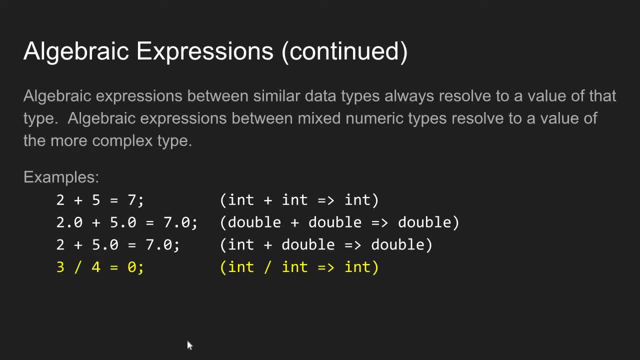 So when we mix ints and doubles, we get double. But here's where this is going to catch you. If I take an integer 3 and divide it by an integer 4, well, 3 divided by 4 is 0.75.. But there is no .7 anything inside an integer. 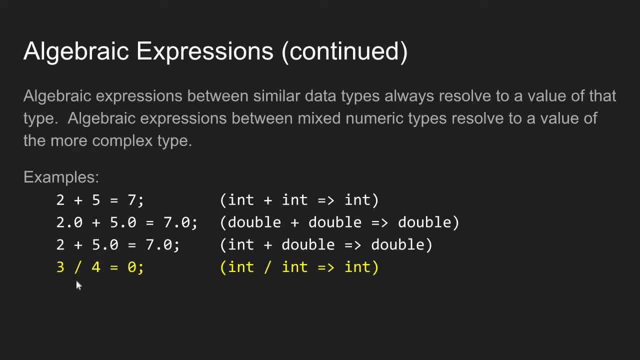 Integers are only whole numbers. So the integer 3 divided by the integer 4 gives me the integer 0. We lose the decimal information. So the one thing we need to look out for when we are doing algebraic operators is that when I am dividing an 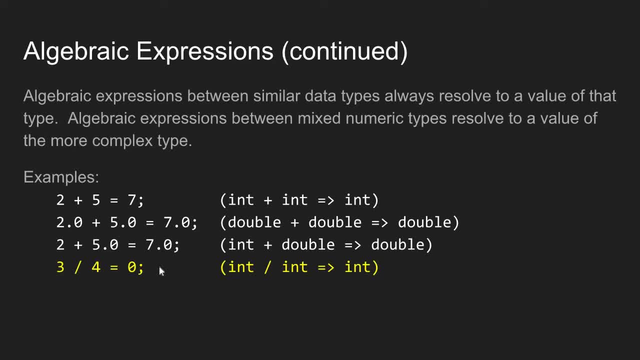 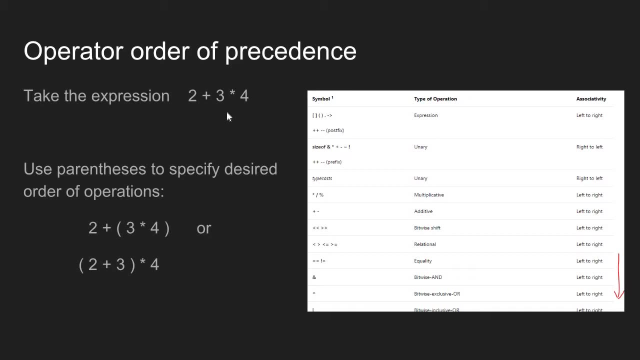 integer by an integer, I will lose my decimal precision in the in the result. So we might have to figure out ways to handle that Something. to think about Operator order of precedence: Now all of the operators in C-sharp have an order in which they are executed. So for example, if I have the expression 2 plus, 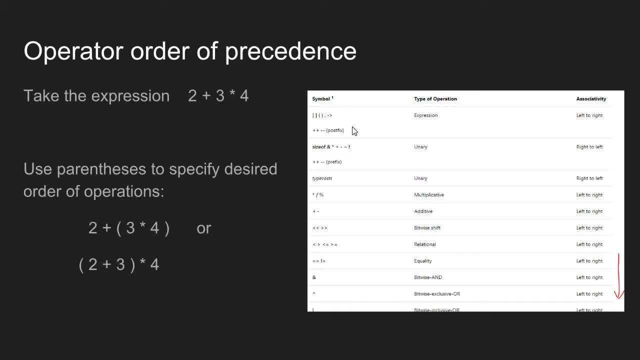 3 times 4,. I can look at a table in a C-sharp table and it will tell me that well, the additive operators plus and minus occur after the multiplicative operators like multiply or divide, And there's many, many more rows on this. 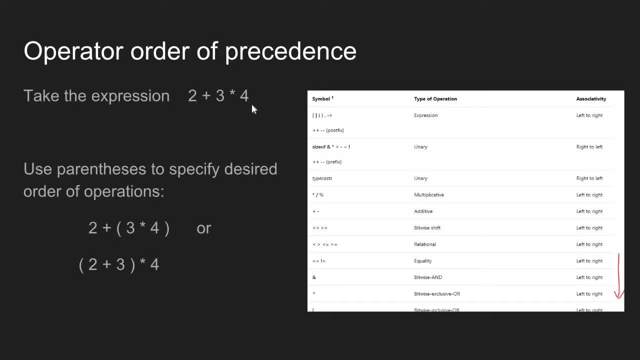 table. If we were to leave this expression to C-sharp, C-sharp would first multiply 3 by 4, then it would add 2.. So there's an order of precedence that it follows, But instead of trying to memorize this large table, we can use parentheses to very 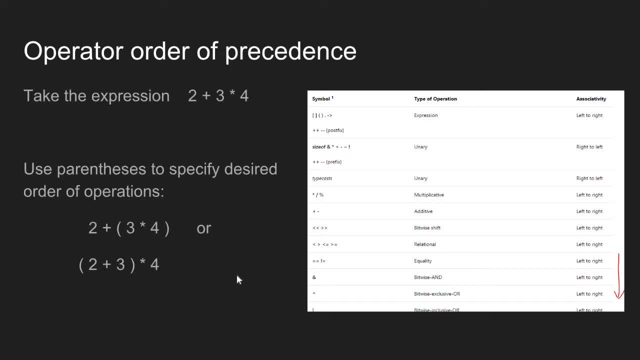 explicitly specify the order that we want our expression to execute. So, for example, if we wanted 3 to multiply by 4, instead of just relying on operator precedence, I believe it is a good idea to specify: Put parentheses around the 3 times 4.. 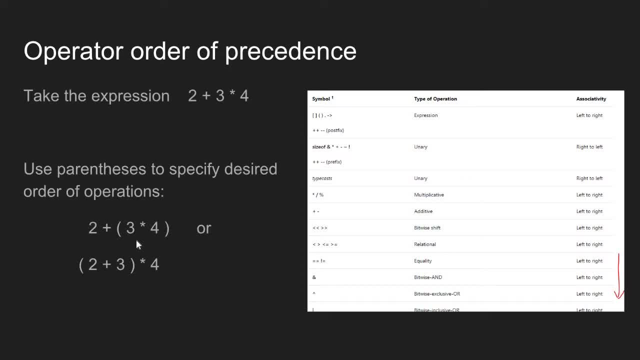 Whenever you use parentheses, the innermost parentheses executes first, and then you work your way out. So if we have more and more sets of parentheses, the innermost execute first and then you work your way out. If I wanted the 2 plus 3 to 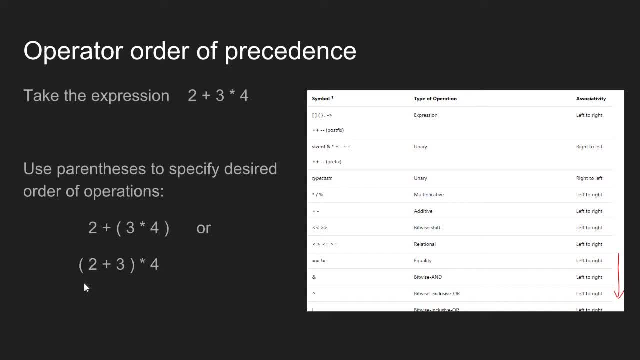 occur before my multiplication, then I could use parentheses here. I would put parentheses around the 2 plus 3, then multiply that quantity by 4.. So the innermost parentheses would execute first. 2 plus 3 would give me the result 5, then 5 times 4 would give me 20.. Alright, I think I'm. 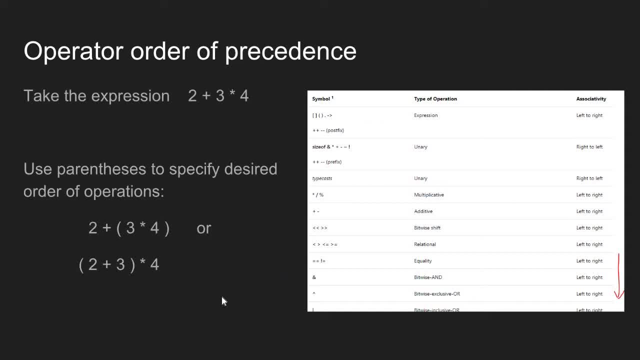 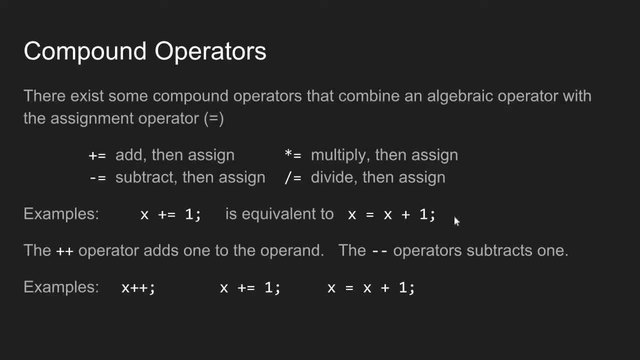 going to make a future video that that shows how you can implement some basic formulas using C-sharp Compound operators. So there are some compound operators that combine an algebraic operator with the assignment operator. These are just short and simple formulas, But if you want to learn more about them you can go to C-sharpcom. 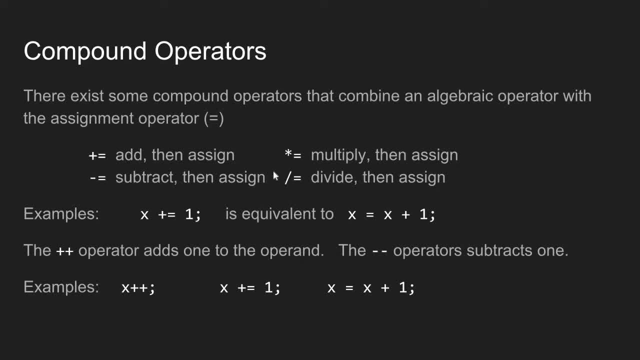 So let's go back to C-sharpcom and we're going to go back to the C-sharp shortcut operators. The four common ones that we should all be familiar with are the plus equals, minus equals, times equals and divided by equals, compound operators. The way these work are: when you see a plus equals, you are you are going to first add the value to the variable, And first you're going to add the value to the variable, then you're going to assign the result of that expression back into the variable. So let me show you an example. 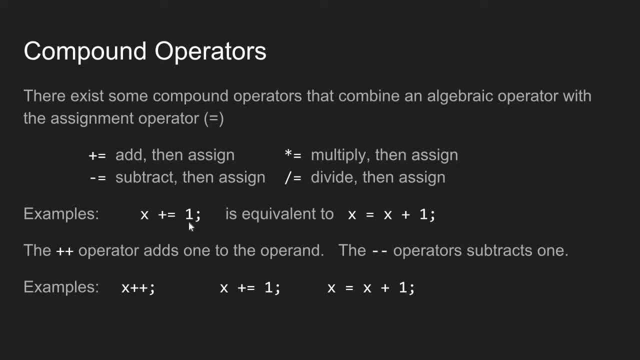 Here I have the expression x plus equals 1.. The plus equals operator is going to take 1, add it to whatever value is already in x, and then we're going to save that result back into x. So we're adding this value 1 into the variable x. 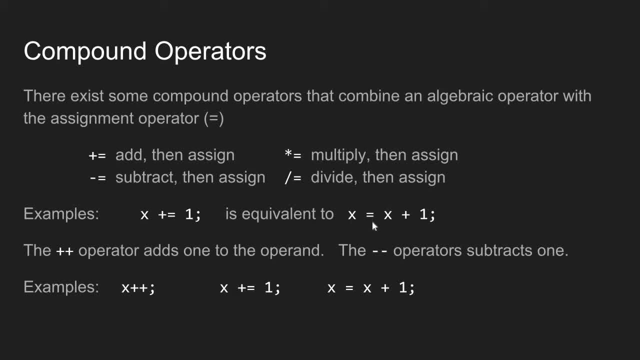 This expression is exactly equivalent to the expression. x is equal to x plus 1.. I'm taking the value 1, adding it into x- the old value of x- and then assigning the result of that addition back into the variable x. I'm updating x with an addition. 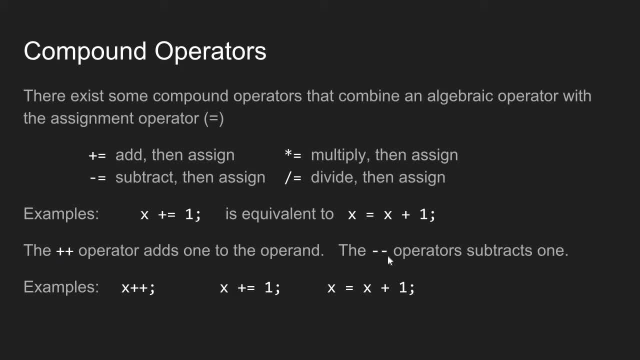 There are two more operators, the plus, plus and minus- minus operators- that take this one step further. If you are adding or subtracting exactly the value 1 from your operand, then the plus, plus or minus minus operators can come into play. So plus- plus operator adds exactly 1 to the operand. 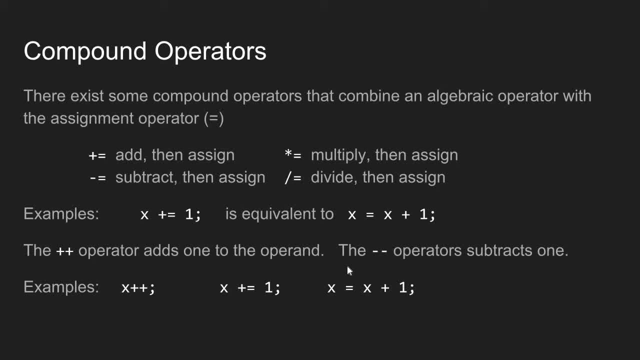 the minus minus operator subtracts exactly 1 from the operand. So for example, x plus plus, the x plus plus operator is going to add 1 into x. So if x is 10, x plus plus means x will now be 11.. 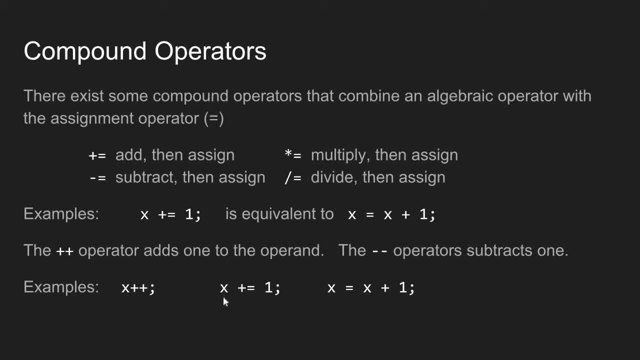 This expression is exactly the same as x plus equals 1, where if x is the value 10,, I'm going to add 1 to 10, which is 11, and then assign that result back into x, And again, both of these are exactly the same as x is equal to x plus 1.. 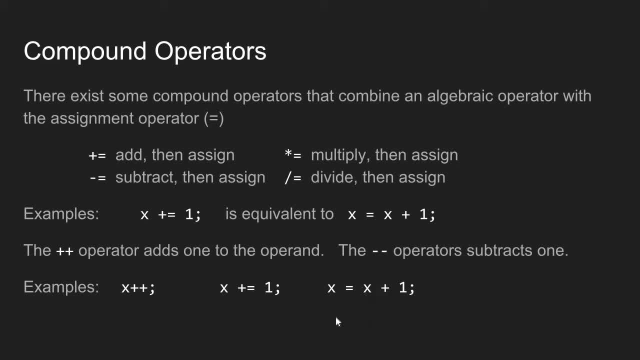 I'm going to take the old value of x, add 1 to it and save the result back into x. These operators are useful shortcut operators and they are used often enough that we should memorize them. We should be familiar with these compound operators. 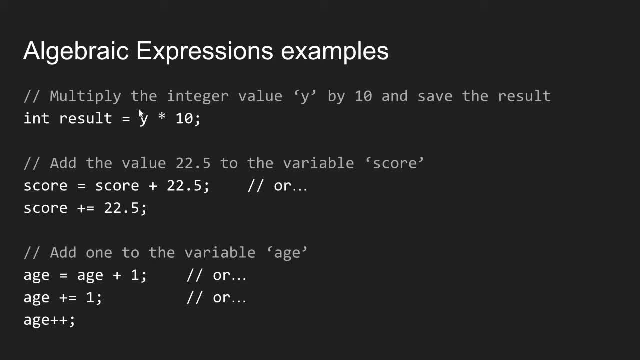 So I'll end the video with just a couple examples here. So let's say we want to multiply. Let's say we want to multiply the integer value y by 10 and save the result. So multiply y by 10, save the result. 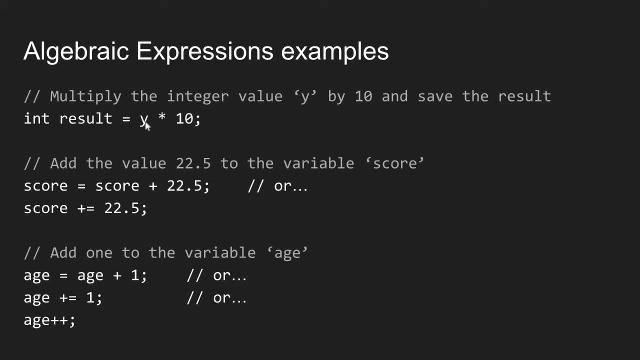 So here I'm going to create the algebraic expression y times 10.. The asterisk is the multiplication operator, And then I'm going to save the result of this expression into some new variable. So I created a variable called result that holds an integer value. 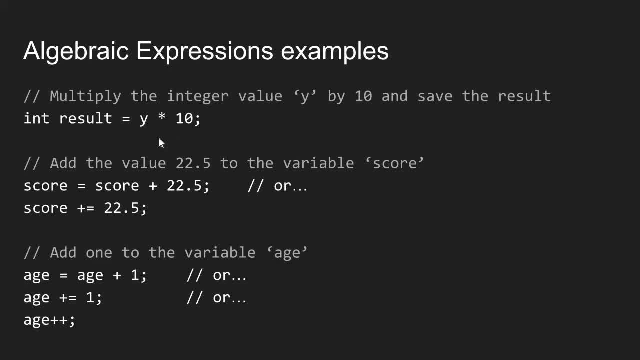 Because y is an integer and 10 is an integer, the result can be saved into an integer variable. Next I have the statement: add the value 22.5 to the variable score. So I want to add a value to an existing variable named score. 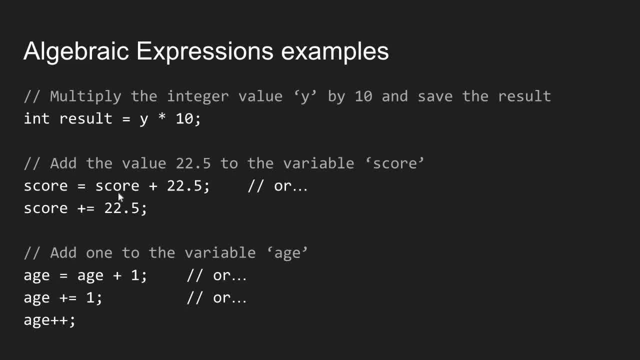 Well, I could do this using the following: expression Score is equal to the expression score plus 22.5.. I'm going to add the old value of score to 22.5 and then save that result back into score. We're updating score with an addition. 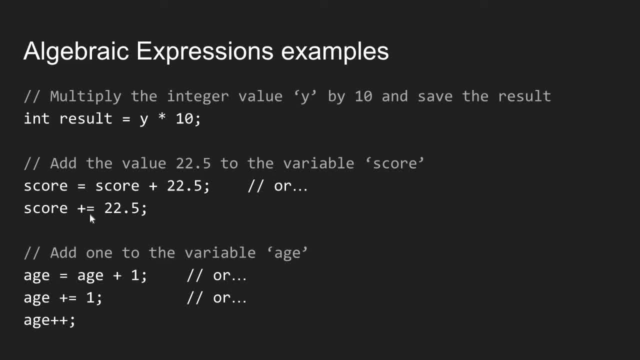 Or we can use the shorthand compound operator plus equals. These do the exact same thing: Score plus equals 22.5.. I'm going to add 22.5 to score and then save the result back into the variable score. And then the final example: I want to add 1 to the variable age. 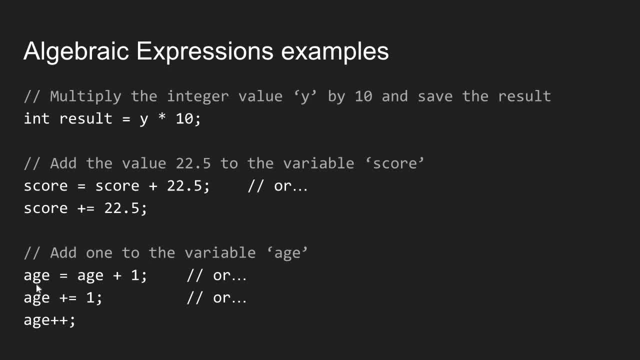 So I'm adding exactly 1.. Well, I can write the expression: age is equal to age plus 1.. I'm going to add 1 to the old value of age and then save the result back into the variable score. So I'm going to add the old value of age to the variable score. 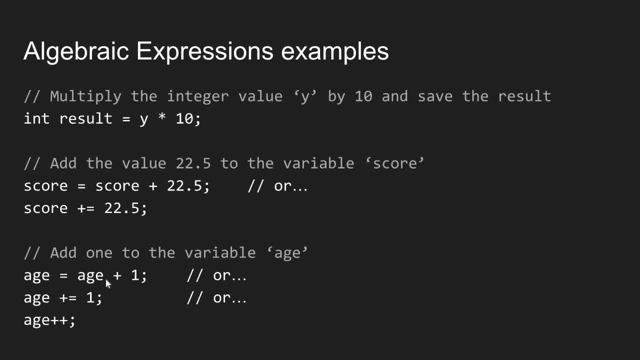 So age is updated with the old age plus 1.. Or I could use the compound operator plus equals. Age plus equals 1.. Here I'm going to add 1 to age and save the result back into age. Or I could use the even further shortcut age plus plus. 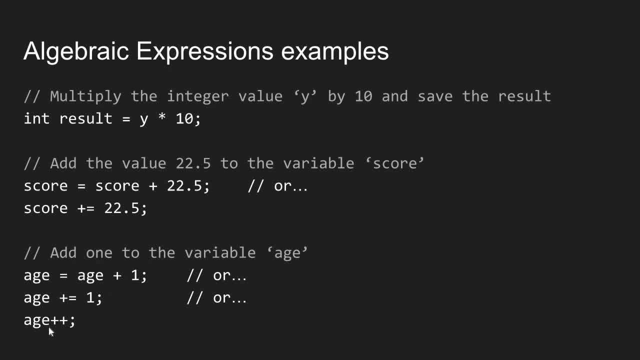 because we are dealing with just the value 1.. Age plus plus will add 1 to the previous value of age. Hope this helps. It's actually relatively easy to hang the whole thing in the Isaiah book. All right, So I just kept it in my tag for now. So if you're going to add anything at the end, let me know in the comments, And if it's not found, just let me know in the comments. Hello friends, in this video we'll be discussing binary operation and its properties. Welcome back students. In this video we are starting with the new chapter, algebraic structure- Very important chapter. So what algebraic structure we going to study under this chapter?